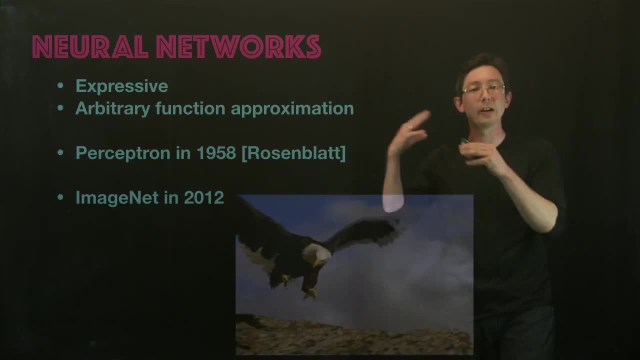 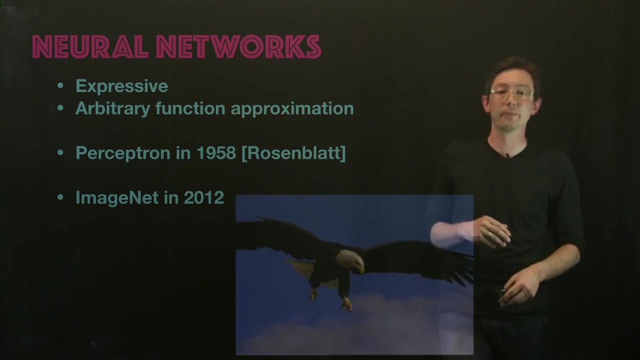 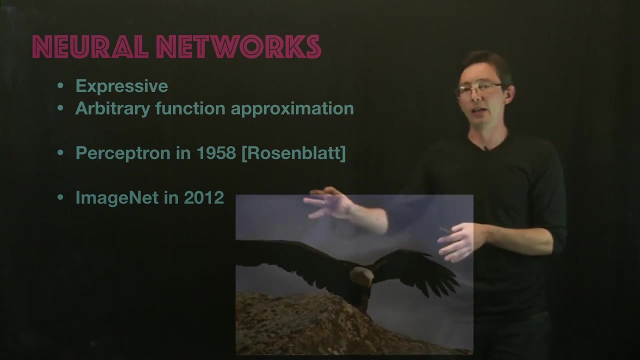 Welcome back. So we're talking about neural networks, which are very expressive machine learning architectures for arbitrary function approximation, And we're talking about the architecture kind of how they work, what the different types are, And what I want to talk about now is why they are having this huge resurgence. Why are neural networks everywhere? 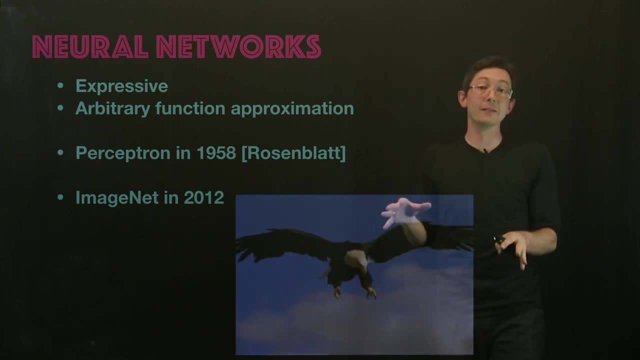 now, when before 2012, they weren't even mentioned in the top 10 algorithms, for example. So something big happened in 2012 that put neural networks back on the map, And I'm going to walk you through, kind of, what that was and what the new capabilities are and where these are going. Okay, So we've 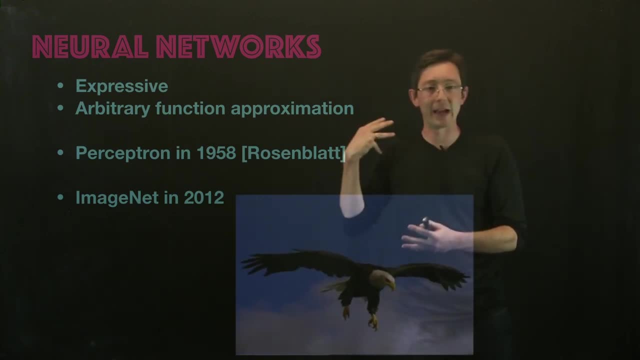 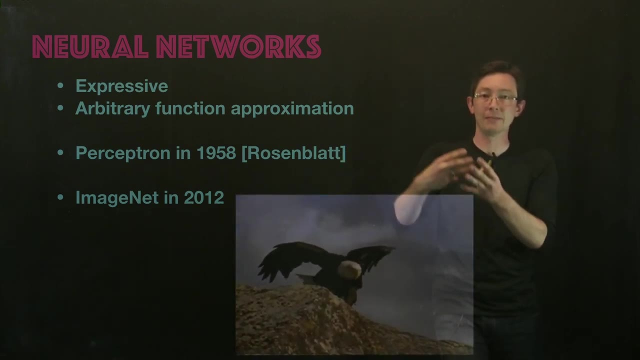 known for a long time, or at least hypothesized for a long time, and this goes back to the neuroscience- that if you had deeper, bigger neural networks- like our brain has a ton of neurons and many, many, many layers of connections- maybe you could get more expressive, better neural networks. 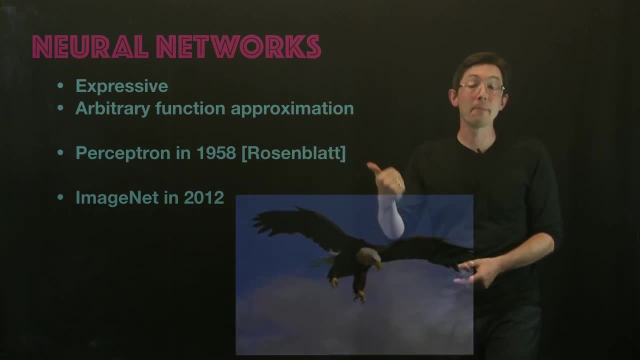 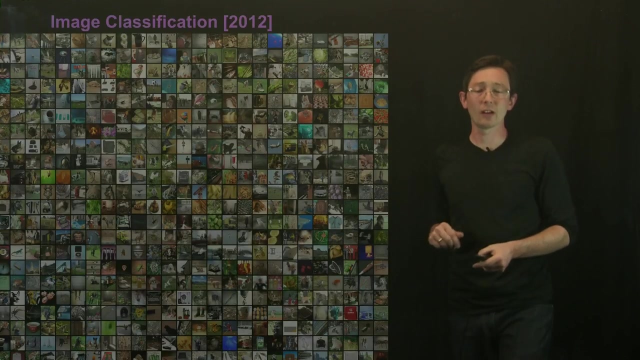 And back in the olden days, we didn't have enough data and big enough computational architectures and good enough algorithms to train these kind of deep, big neural networks, And so that's really what changed in 2012 with this ImageNet data set that I'm going to tell you about. 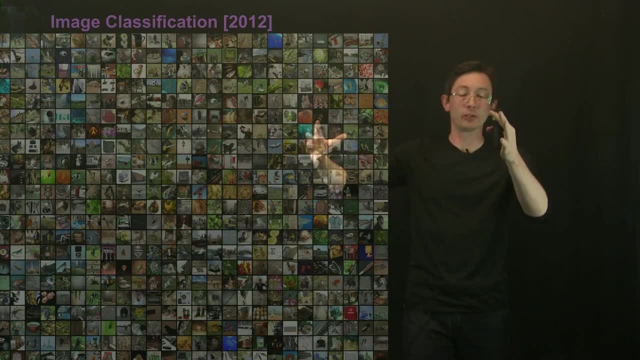 So what you want to do is train this big deep neural network, And so what you want to do is train this big deep neural network And so neural network, but there's a lot of degrees of freedom, There's a lot of free numbers. 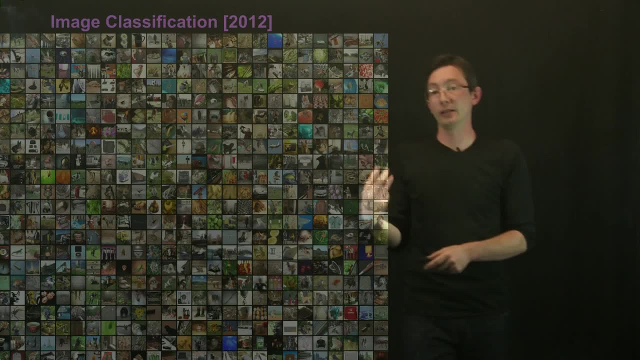 free parameters you have to tune, and so you need a lot of training data to fit those models. In addition, if I want to be able to reliably know what is a dog and how is that different than a cat and how is that different than a pickup truck, I need a lot of examples of 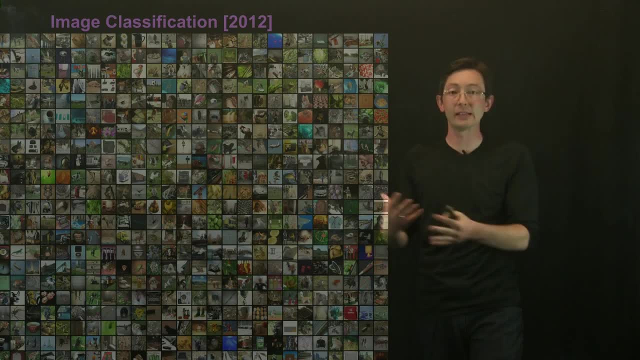 all of those labeled data And this was a very expensive labeled data set in 2012, this ImageNet data set with millions of labeled images, So you might have thousands, thousands of images of a dog that are labeled dog and thousands of images of cats and trucks, and 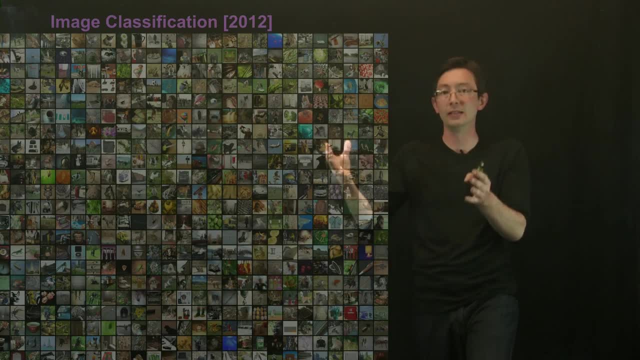 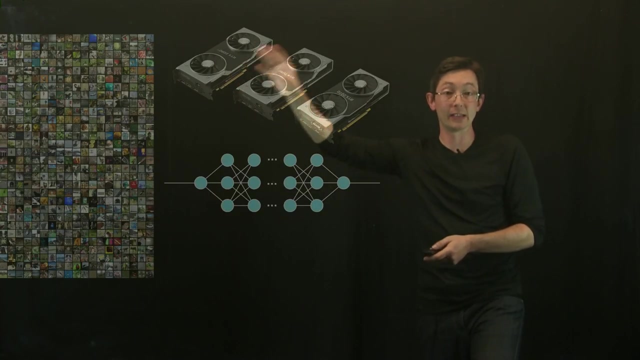 cars and broccoli and everything you can imagine. everything you've seen practically is in this ImageNet database labeled images, And that in combination with increasingly powerful computational algorithms- so kind of GPU, graphics, processing unit computers- you can do very, very massively. parallel computations on multiple cores allowed us both the computational 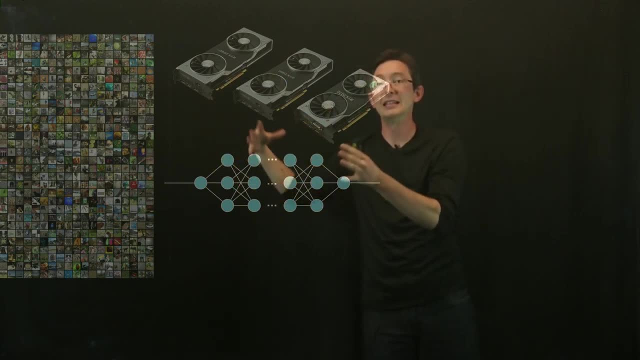 hardware, the architecture, the labeled data to start training these deep, more expressive networks. And so that was kind of the birth or the rebirth of deep learning, And since then it's taken over many, many, many aspects of our machine learning in our daily lives. 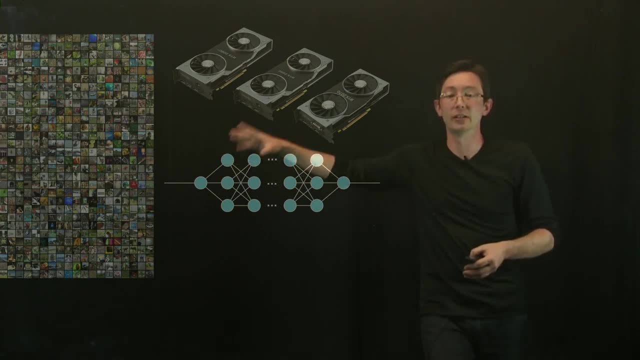 from Alexa and Siri to image classifying, And I'll also point out that there is a huge development of open source software. so the industrial investment by big tech companies billions of dollars of research and development of open source software and kind of community-driven research and software, has really also contributed. 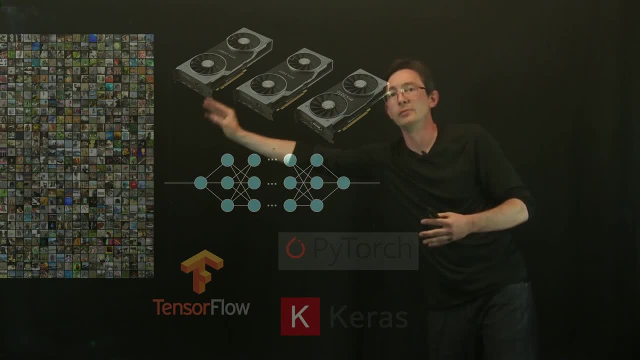 to driving this. So you have your big labeled data: unprecedented volumes of quality data, massive and increasing architectures for processing this data and training these algorithms which facilitate deep, deeper, larger architectures. And the software is getting much better to train this all. So in the olden days you'd have to program the framework to train these. 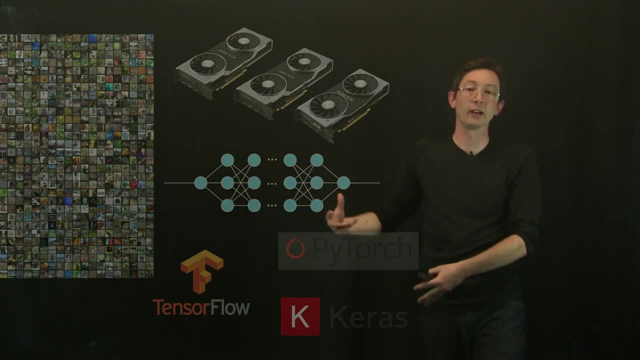 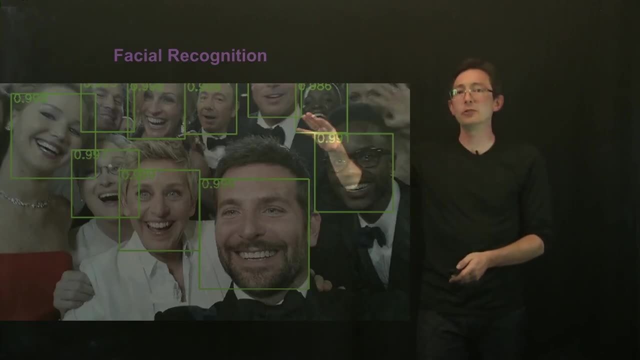 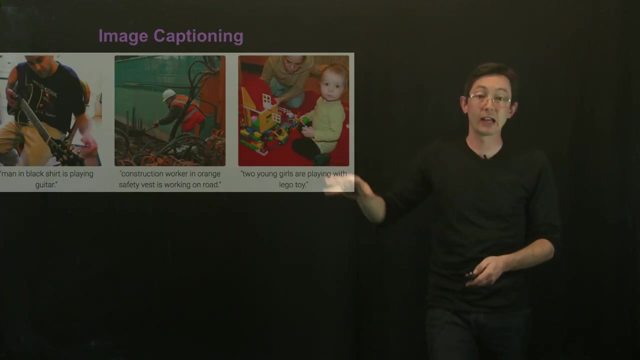 algorithms, And now with TensorFlow and PyTorch and Keras, it's much, much easier to do this with your data, with new data, Okay. And so this is ubiquitous. It's everywhere in facial recognition surveillance, image captioning- This is kind of incredible. You can actually label images. now, This was you. 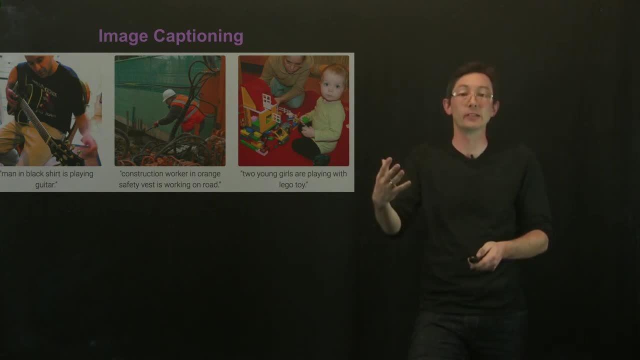 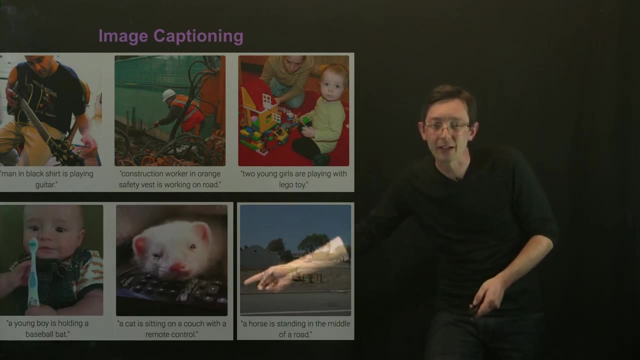 know, even a decade ago, we thought this might be impossible. This is something only humans can do. but that's not true. now You can image caption, Not always perfect, You know, this is a cat sitting on a couch with a remote control. Not really. 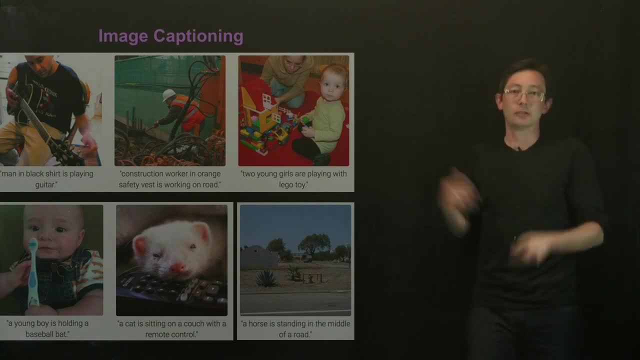 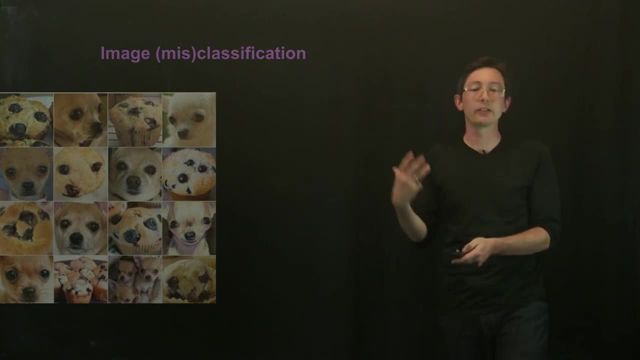 This was one of my favorites: A horse standing in the middle of a road. Where's the horse? But still pretty good. Of course, you know, images are not trivial. They're still canonical things that machines get confused about. I love the- you know- Chihuahua blueberry muffin. It's easy for. 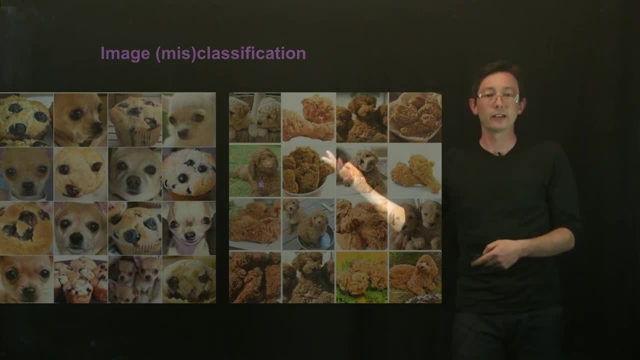 us to tell. Or is it? Fried chicken dog is fun, But overall the performance is getting, you know, at or above human-level recognition in a vast array of tasks, especially in the image recognition, natural language processing, speech recognition, things like that. 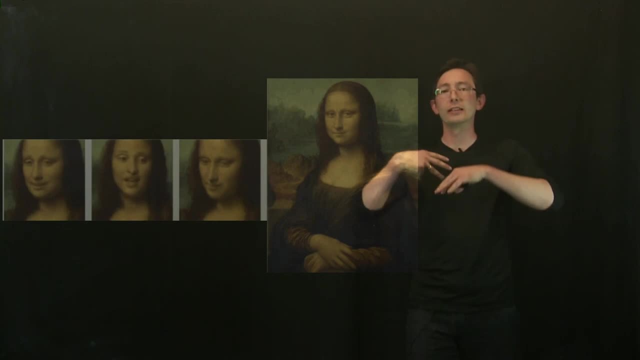 This is pretty cool. This was pretty recent- where a set of researchers are using these generative networks, these GANs, to start doing, you know, generative models. So from one picture of the Mona Lisa, they were able to make these very realistic, lifelike sequences. 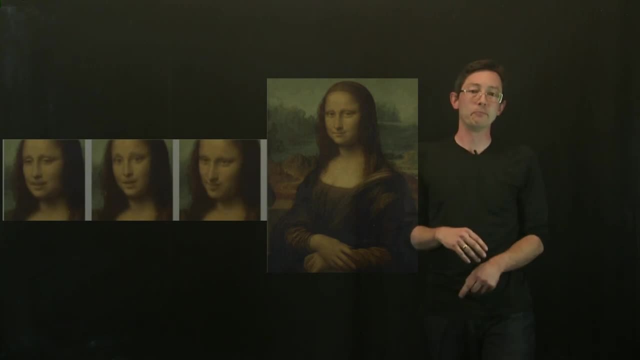 that look like she's speaking and interacting in the real world. So these generative models, you might have seen them If you put a picture. you know there's websites. you can upload a picture and it'll make it look like Van Gogh painted it. That's this kind of technology, But the implications are. 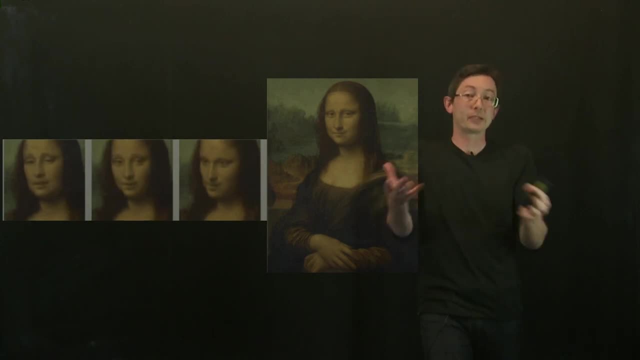 pretty profound. I mean, this is going to change. perhaps you know our society at the core. What if you can't trust the news you're seeing, because people can generate videos that look just as real as the real world? What if you can't trust what your politicians 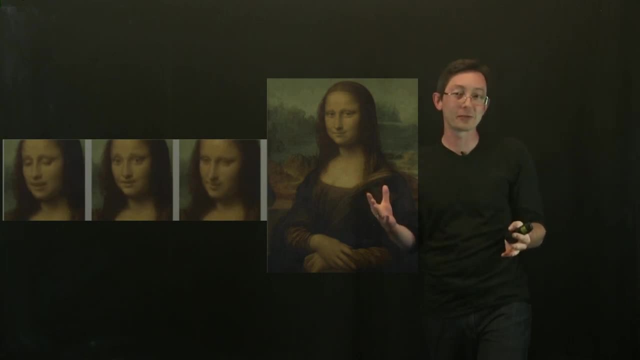 are saying: Maybe you couldn't trust what your politicians were saying already, but what if you don't even know if it was them saying it? I mean, this changes a lot. So there's a bunch of really exciting applications. Maybe I can. 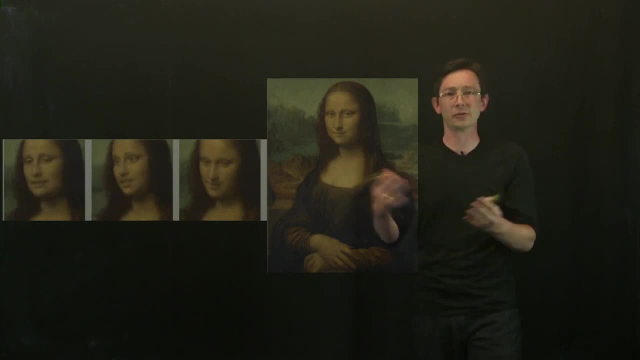 generate new airfoil designs or new automotive designs or new engineering designs in general that I've never seen before. There's really cool applications of that, But there's also serious kind of concerns that we should be thinking about in these generative models. So again, neural networks in general can be very expressive, But you